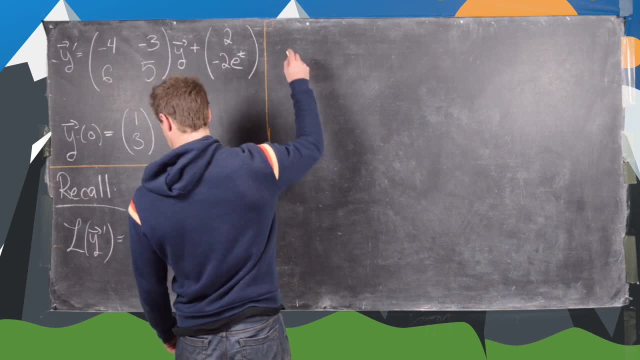 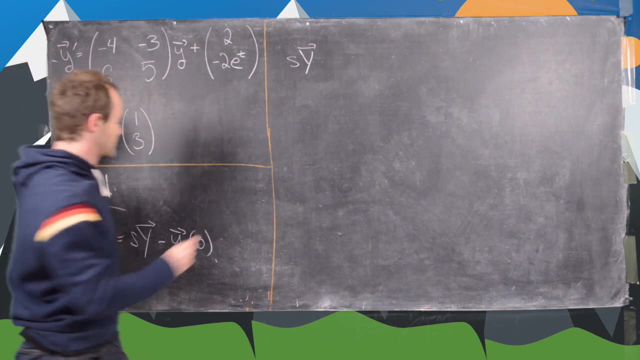 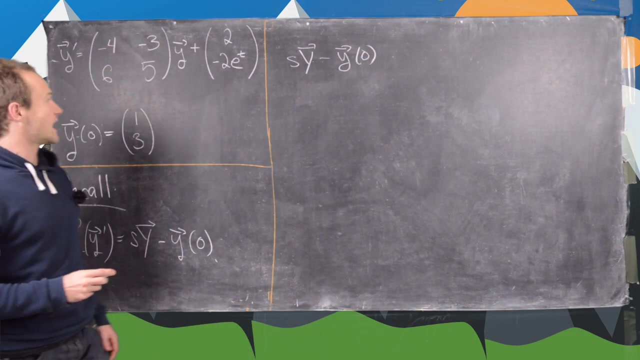 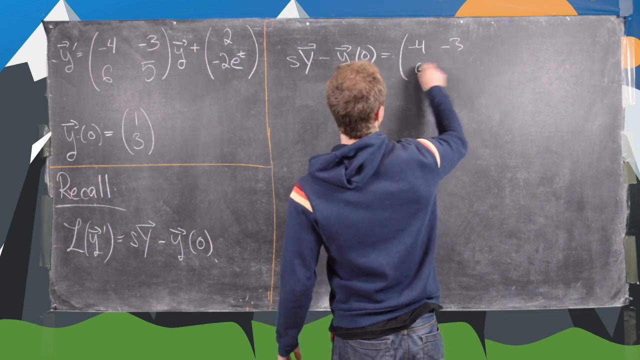 Sorry, this differential equation. So that's going to give us s times y, capital vector. So that would be like this part minus y, evaluated at 0.. So there, we've done that And now we have. this is the matrix minus 4,, minus 3,, 6, 5.. 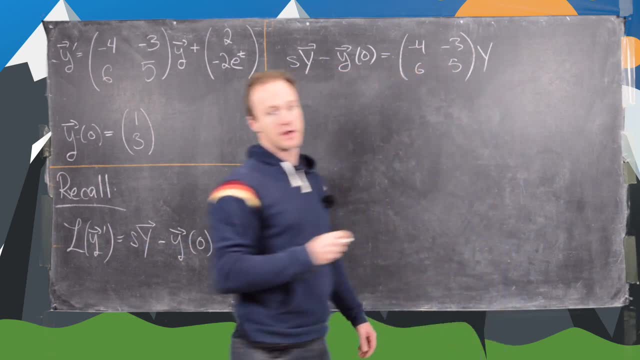 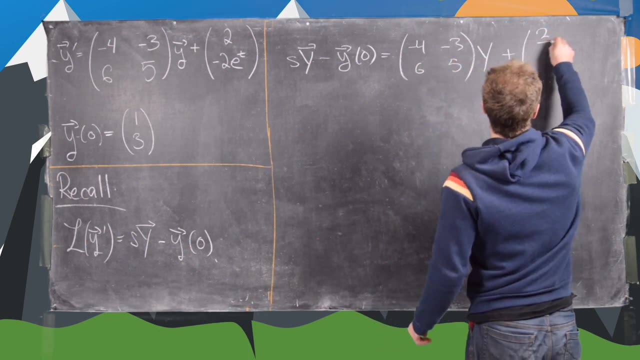 Now we apply the Laplace transform to this, giving us capital y. We're using that notation. Now we apply the Laplace transform to this vector valued function. So we get 2 over s for the first component, because the Laplace transform of 2 is 2 over s. 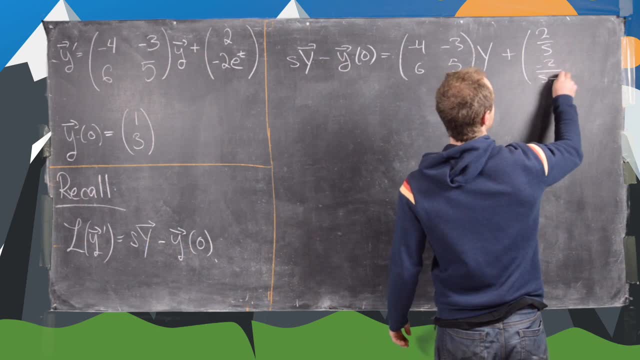 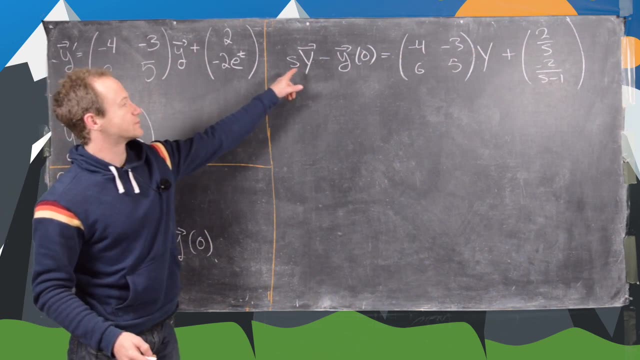 And then for this guy we get minus 2 over s, minus 1.. So that's the Laplace transform of e to the t. Okay, now we're good. Now what we'll do is we'll replace this initial condition with what we know it is. 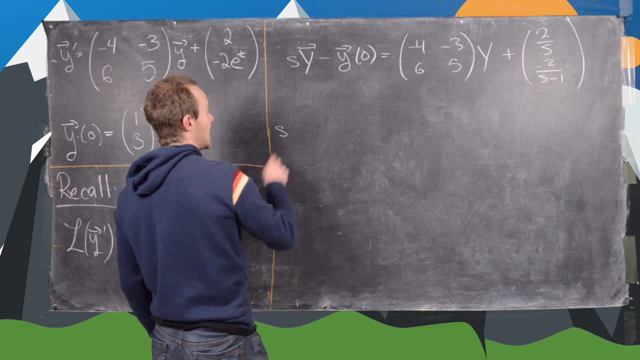 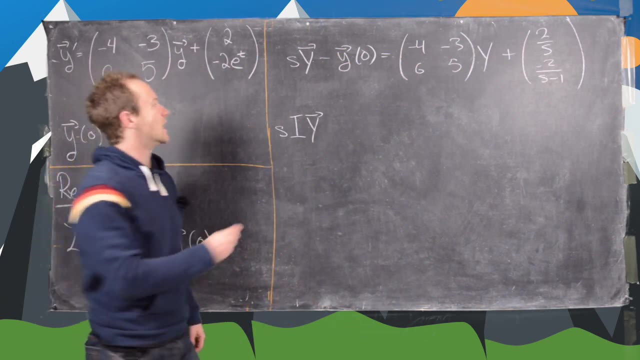 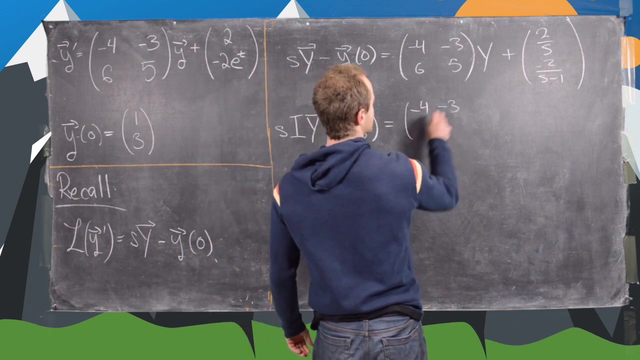 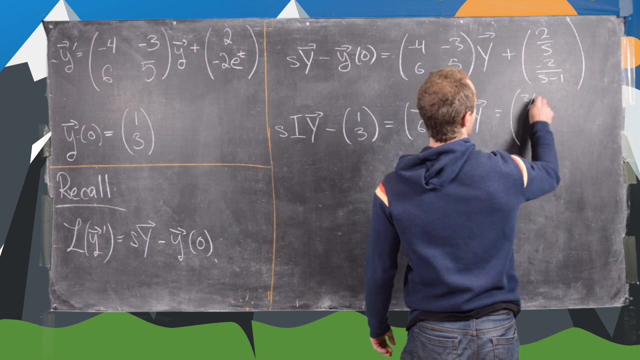 So that's going to give us s times. Now I'm going to write this as the identity matrix times y, in order to make it look like this guy over here: Minus 1, 3 equals Now this matrix minus 4, minus 3, 6, 5 times y vector equals this: 2 over s minus 2 over s minus 1.. 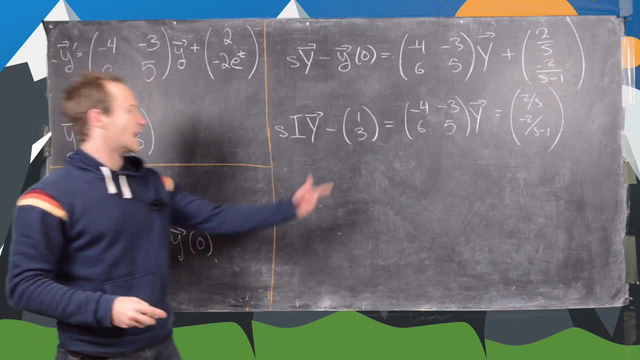 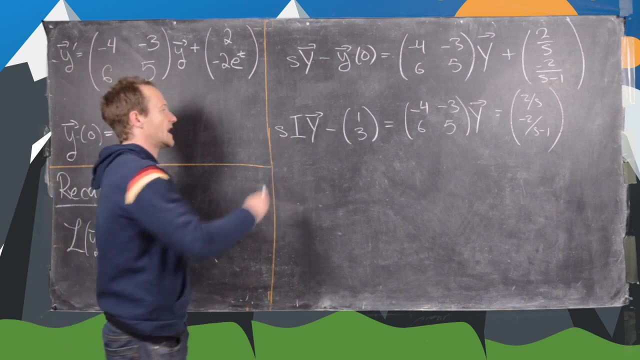 So that's what we have. Okay, now I'm going to move this to the right-hand side and this term to the left-hand side. And so, notice, as I move this term to the left-hand side, I'm going to add these matrices: 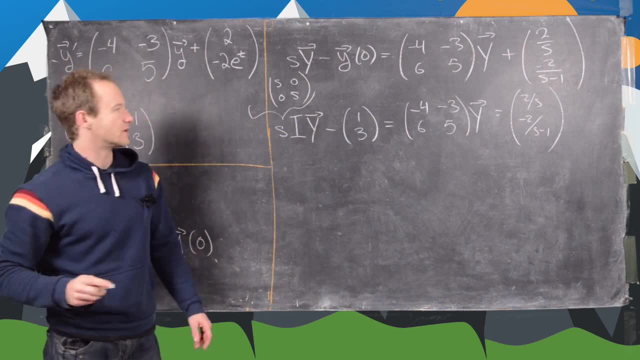 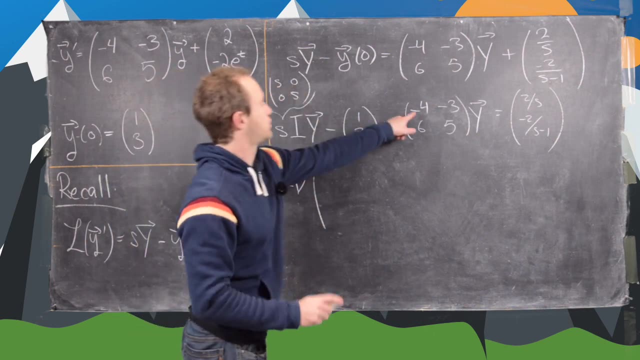 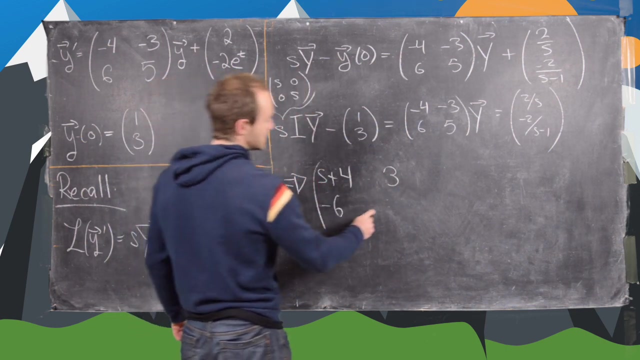 So notice, this is the matrix: s 0,, 0, s like that. So that's going to give us the following: So that will give us s plus 4, and then 3.. And then here we have minus 6, and then s. 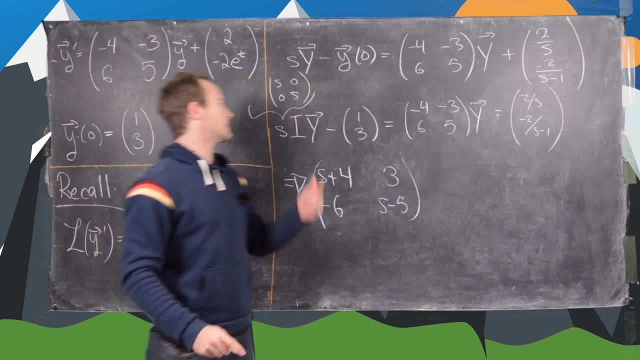 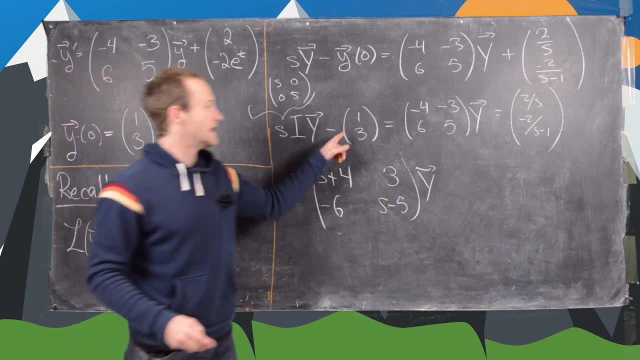 Minus 5.. So that's what we get from subtracting this matrix from this matrix, And then we have that as all multiplied by y. Okay, great. Now when we move that over, we'll have the following vector: So we'll have 2 over s plus 1.. 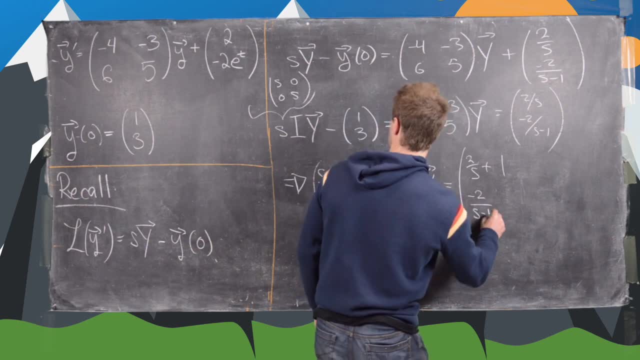 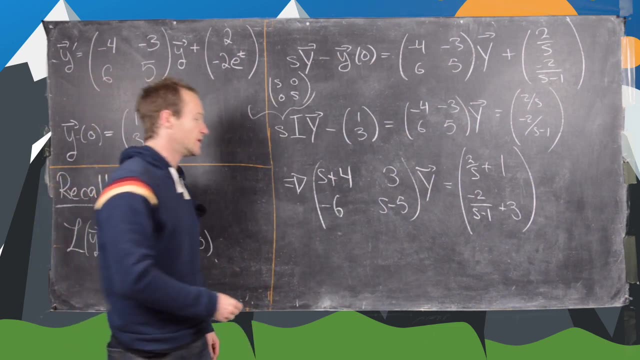 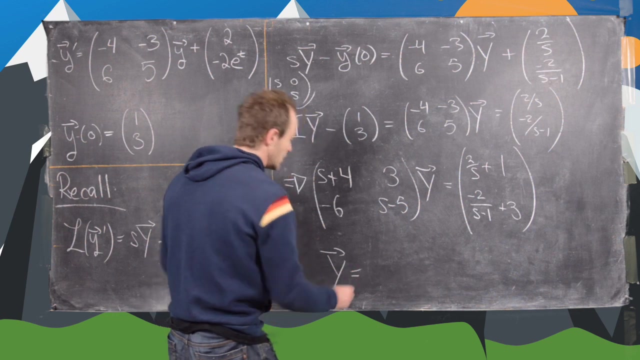 And then we'll have minus 2 over s, minus 1 plus 3.. Okay, good, So the next thing that we can do is Say that y, in other words the Laplace transform of our solution, will be given by the inverse of this matrix times this vector. 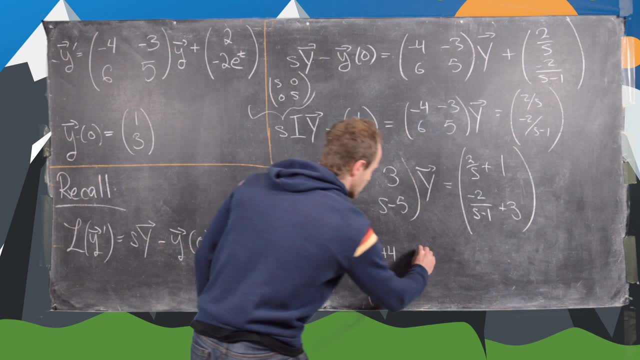 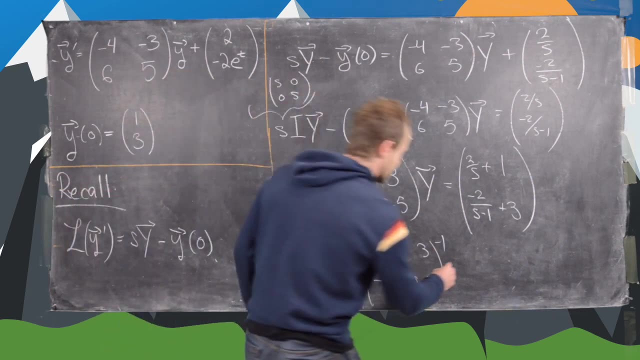 So let's write that down. So that's going to be s plus 4, 3 minus 6, s minus 5, inverse times this vector: 2 over s minus 1, minus 2 over s minus 1 plus 3.. 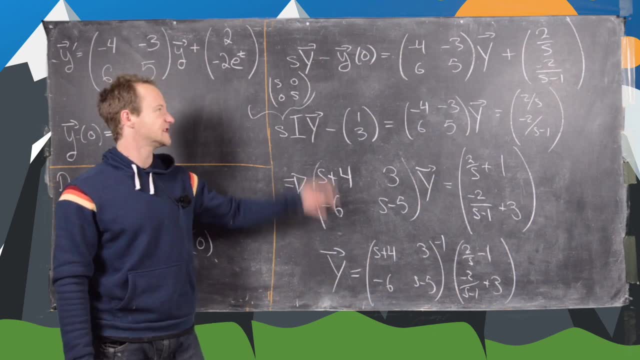 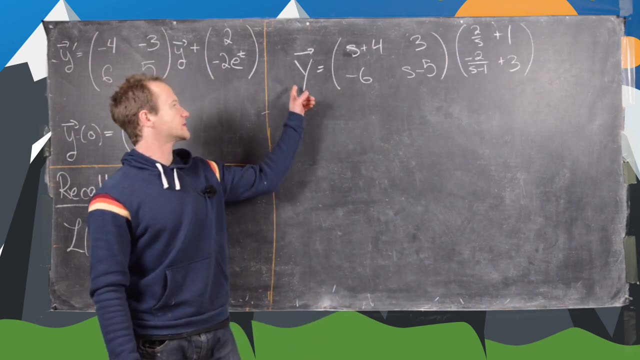 Okay, good, So now I'll clean up the board, I'll move this part to the top and then we'll find our final solution. Okay, so, let's see, I move this up from the bottom, So we have: y equals the inverse of this matrix times this vector. 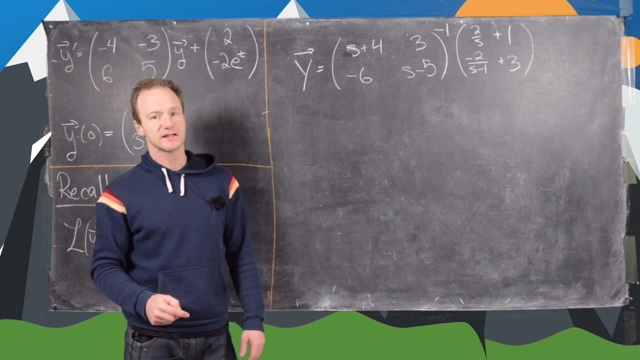 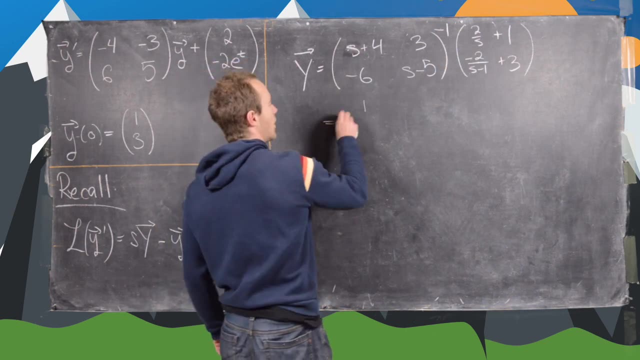 So let's see if we can calculate the inverse of this matrix pretty easily. So notice it's going to be 1 over the determinant. So notice the determinant will be ad minus bc, So it'll be 1 over s plus 4 times. 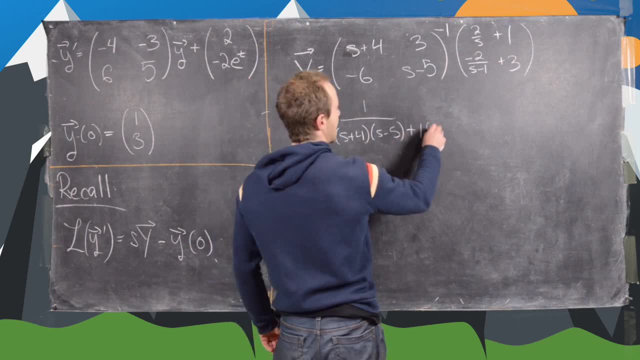 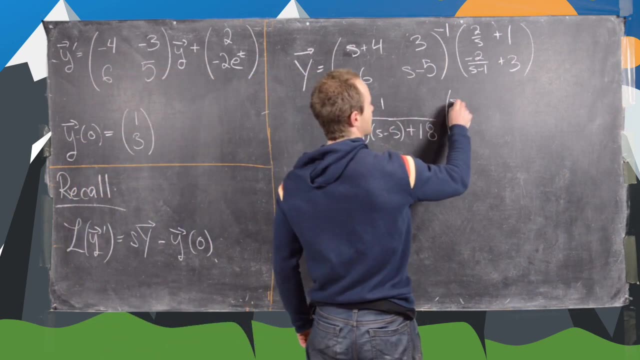 s minus 5. And then plus 18.. So that's what we get for that determinant. And now we need to switch a and d, So that'll be s minus 5, s plus 4. And then negate b and c. 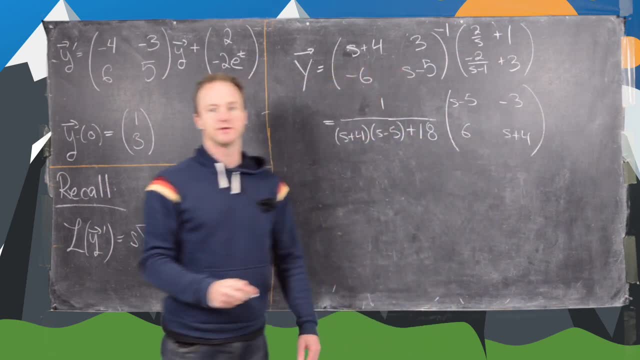 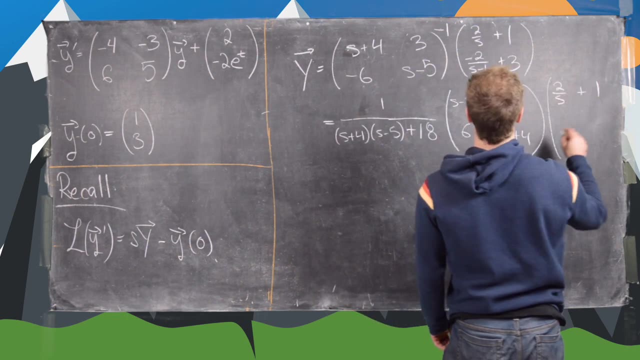 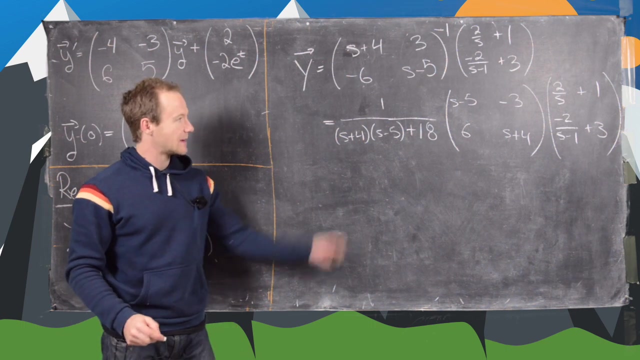 So that'll be minus 3, 6.. So there I use the formula for the inverse of a matrix, And now we have 2 over s plus 1 minus 2 over s minus 1 plus 3.. So we're left with something like that: 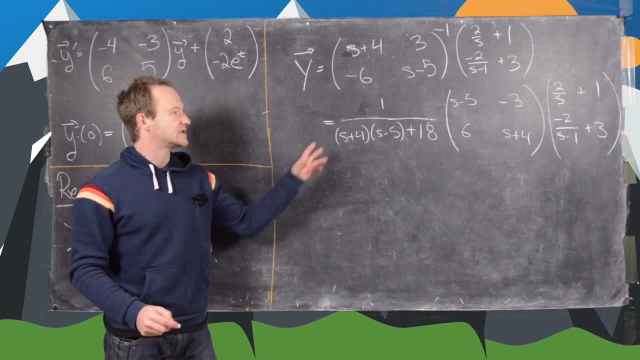 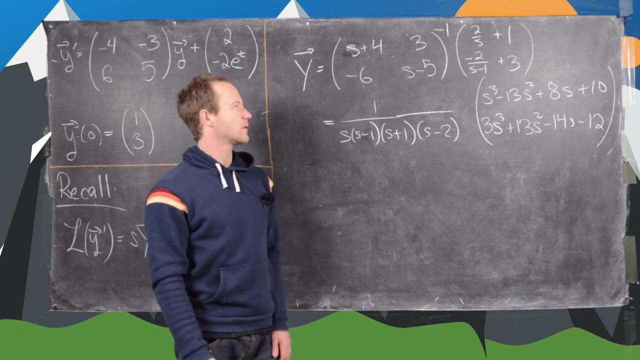 So at this point it's just like a little bit of arithmetic to combine this together into one vector equation. So let's see if we can do that pretty easily. Okay, so there we've got that. After multiplying out the inverse of this matrix with that vector, we get this big thing.